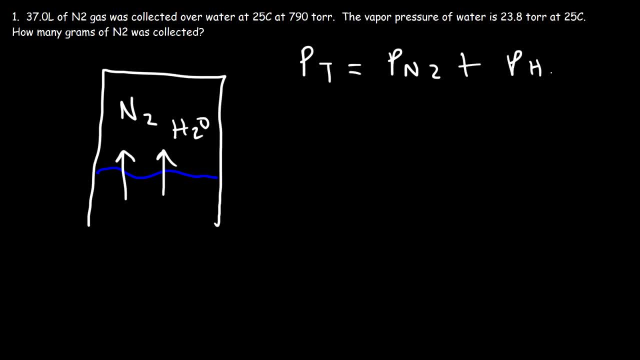 We have N2, and we have water, So you need to take into account the pressure that water exerts. As long as you do that, then you're fine. So we know the vapor pressure of water, which means we can calculate the partial pressure of nitrogen. 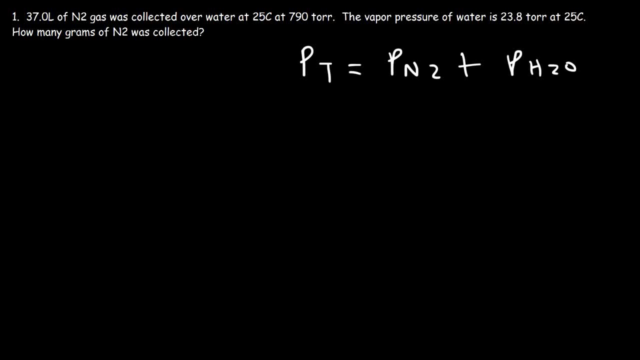 That's the first thing you should do in a problem like this. In this example, the total pressure is 790.. And this term the vapor pressure of water, that's 23.8.. So therefore, the partial pressure of N2 is just 790 minus 23.8.. 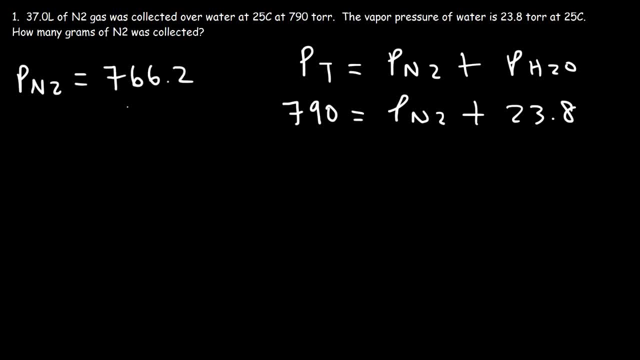 And so that's 766.2 Torr. So now that we have the partial pressure of N2,, we can use the ideal gas law equation to calculate the moles of N2, which can help us to calculate the mass of N2.. 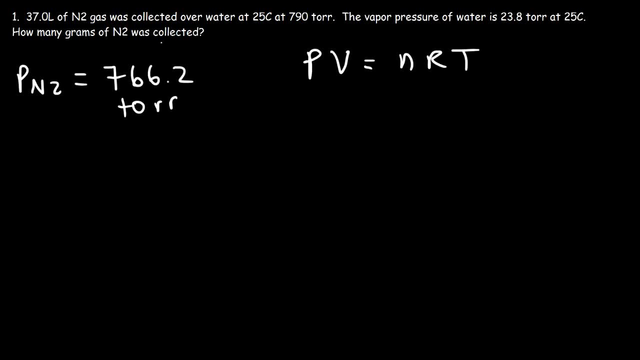 So PV is equal to NRT. Now we need to convert this to ATM. So to do that we need to divide it it by 760.. So 766.2 divided by 760, that's about 1.008 ATM. 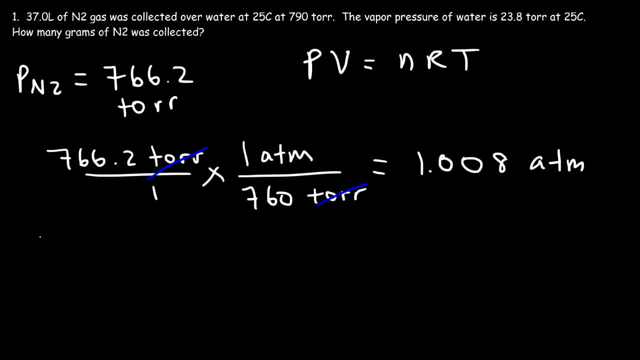 So now let's use this formula. So let's replace P with 1.008, and V is 37 liters. We have that here. Our goal is to calculate N, R is .08206, and the temperature is going to be 25 C plus 273,. 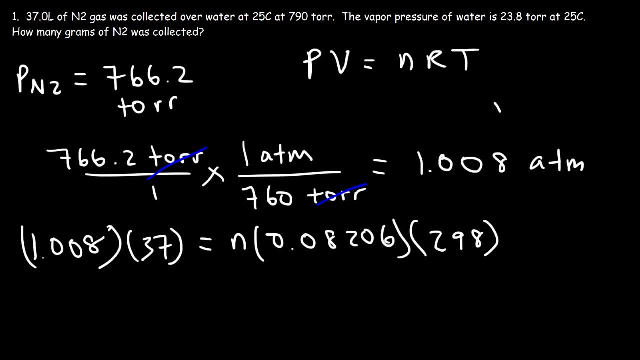 so that's 298 Kelvin. Don't forget to open the calculator. Always use the Kelvin temperature in this equation. So N is 1.008 times 37, divided by .08206, and then divide that result by 298.. So it's going to be 1.525 moles. 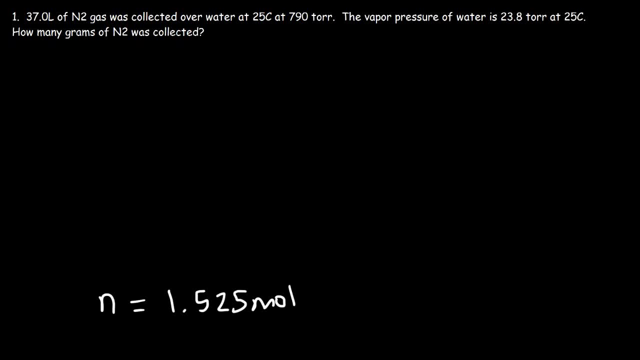 Now the last thing we need to do is convert moles into grams. Now, nitrogen has an atomic mass of 14.01, so we need to multiply that by 2 to get the molar mass of N2.. So that's going to be 28.02 grams. 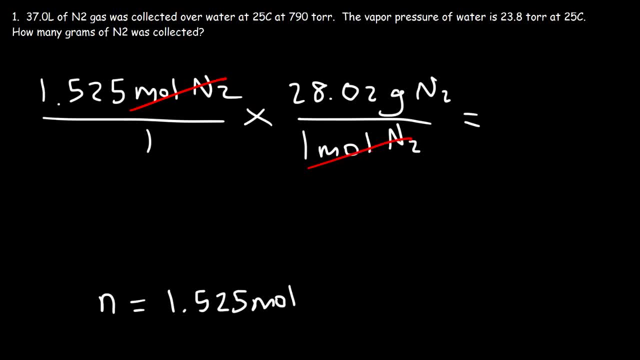 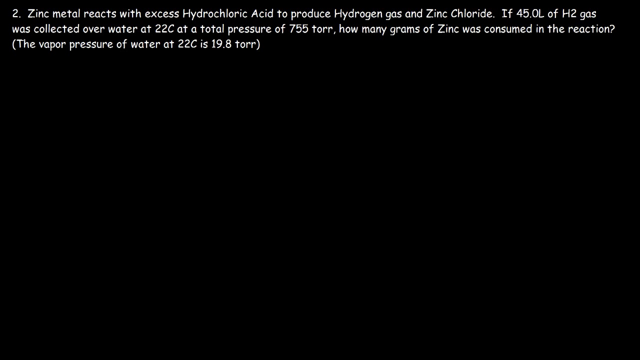 Okay, Great, And so the molar mass, or rather the mass, is 42.7 grams of nitrogen gas. So this is the answer. Let's try this problem. Zinc metal reacts with excess hydrochloric acid to produce hydrogen gas and zinc chloride. 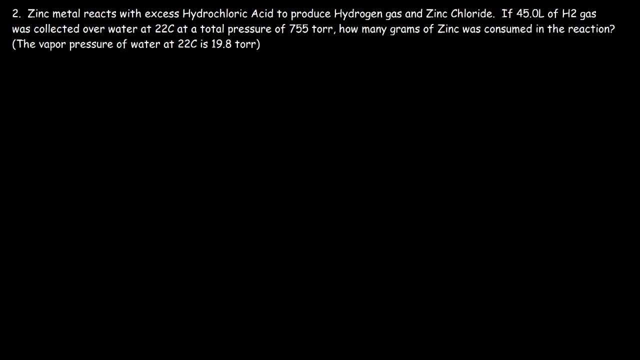 So if 45 liters of H2 gas was collected over water at 22 Celsius at a total pressure of 755 Torr, how many grams of zinc was consumed in the reaction? Well, let's write a balanced reaction. So zinc plus hydrochloric acid is going to produce H2, hydrogen gas and zinc chloride, which is ZnCl2.. 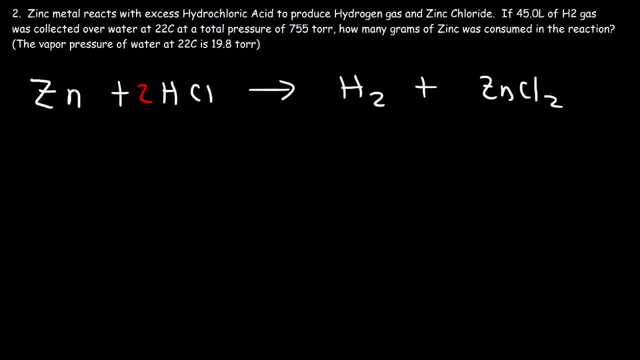 So to balance it, all we need to do is put a 2 in front of HCl, and it's now balanced, So we can put a 1 in front of everything else. Now the first thing we need to do is calculate the partial pressure of H2.. 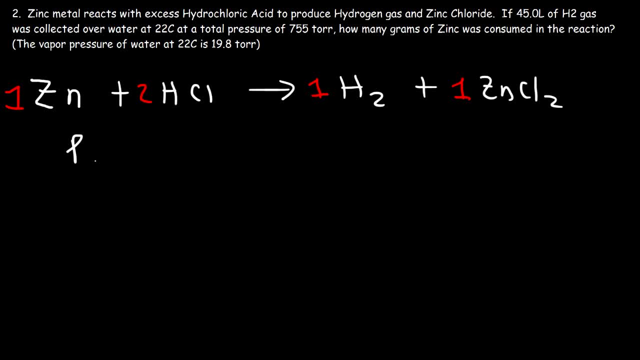 The only gases that we have, or the only substances that exist above the water, is hydrogen gas. it's collected over water plus the water. So we need to calculate the partial pressure of H2.. So we need to calculate the partial pressure of H2.. 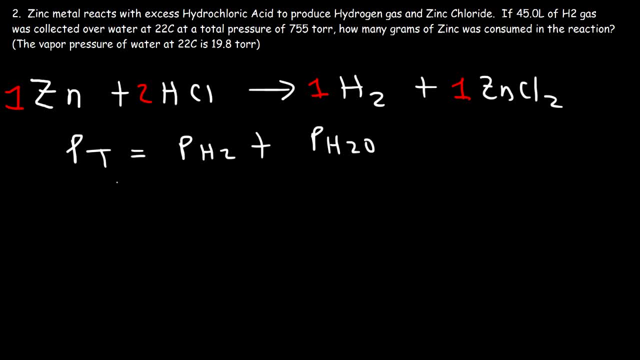 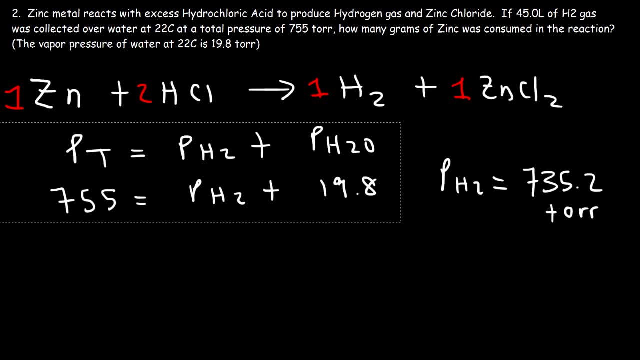 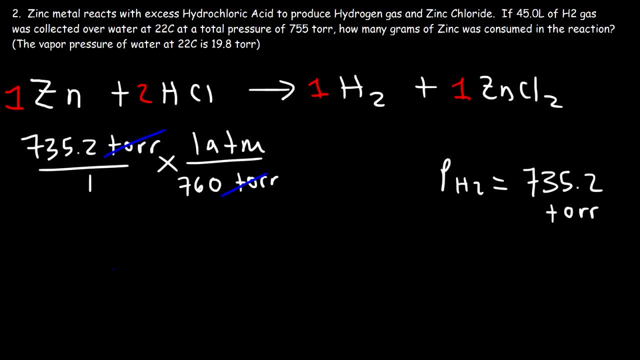 735.2 divided by 760.. is- let's get rid of this- 0.9674 atm. So now we can use this to calculate the moles of H2 that was produced. So let's use the ideal gas law equation: PV is equal to nRT. 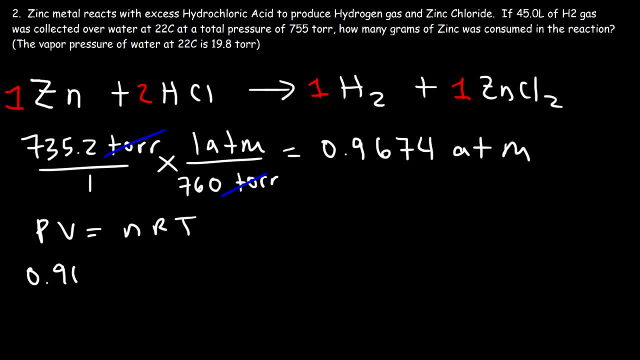 So P is 0.9674,, the volume V is 45 liters, R is 0.08206, and the temperature is going to be 22 plus 273, which is 295 Kelvin. So let's multiply 0.9674 times 45, and then let's 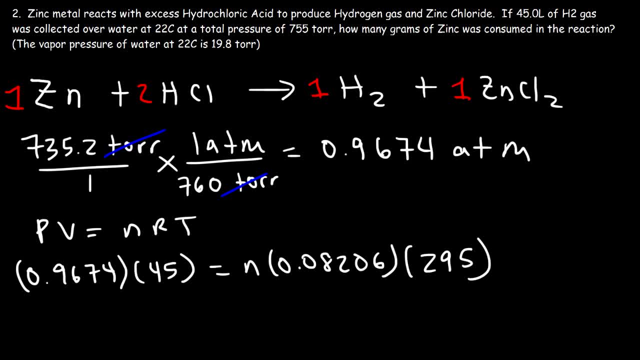 divide. So P is 0.9674 divided by 0.08206, and then take that result, divide it by 295.. So n is equal to 1.798 moles of H2.. Now that we have the moles, 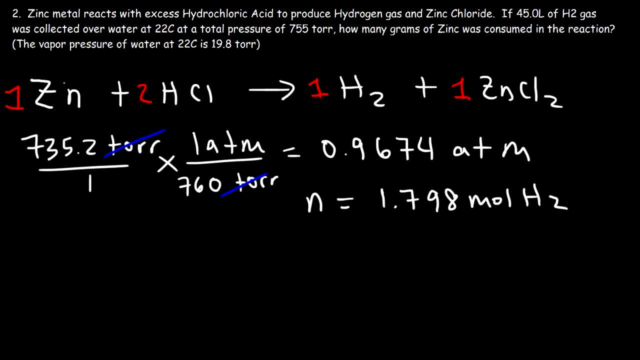 what we need to do is convert it to the moles of zinc, and then we can convert that to the grams of zinc, And that will tell us how many grams of zinc was consumed in a reaction. So let's start with 1.798 moles of H2.. Now the molar ratio between these two substances. is 1 to 1.. So, for every mole of H2 that's produced, 1 mole of zinc is equal to 1.798 moles of H2.. So what we need to do is take our answer, 1.798, and multiply it by 65.39.. 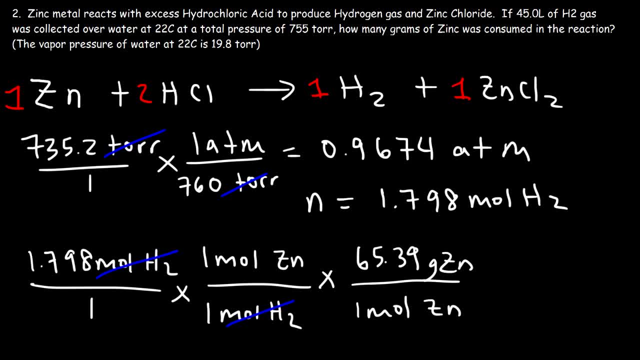 So it's 117.39 moles of H2.. Now we need to take our answer- 1.798 moles of H2, and multiply it by 65.39.. So it's 117.39 moles of H2.. 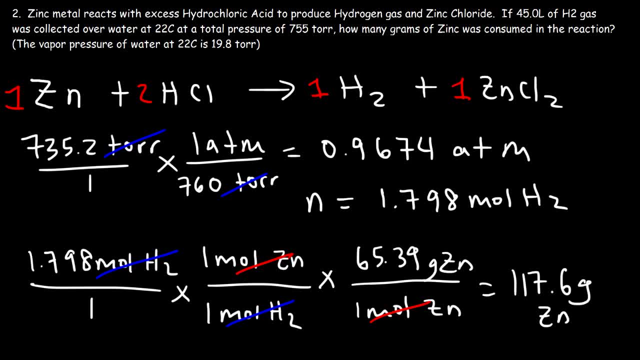 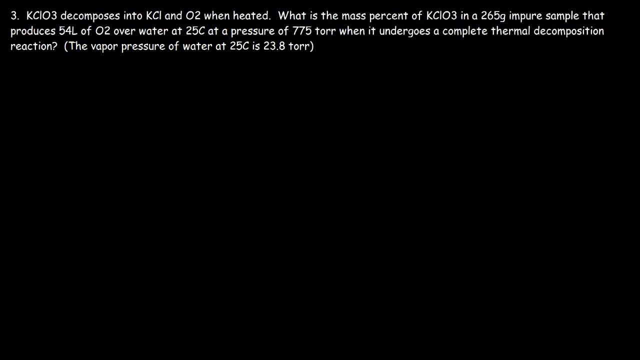 So that's the mass of zinc that was consumed in this reaction. So this is the last question that we're going to go over in this video. KClO3 decomposes into KCl and O2 when heated, So let's write a balanced reaction. 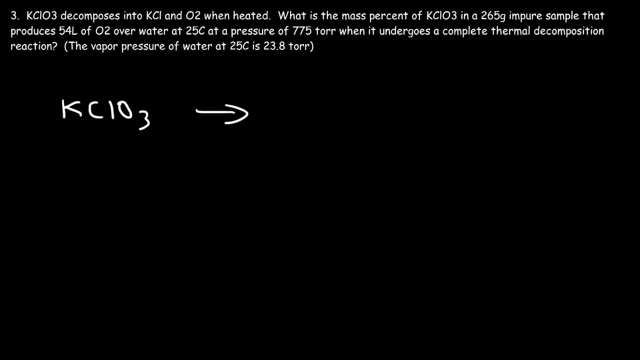 So we have potassium chlorate and it decomposes into potassium chloride and oxygen gas. Now we're going to write a balanced reaction. So we have potassium chloride and it decomposes into potassium chloride and oxygen gas. Now we have three oxygen atoms on the left and two on the right. 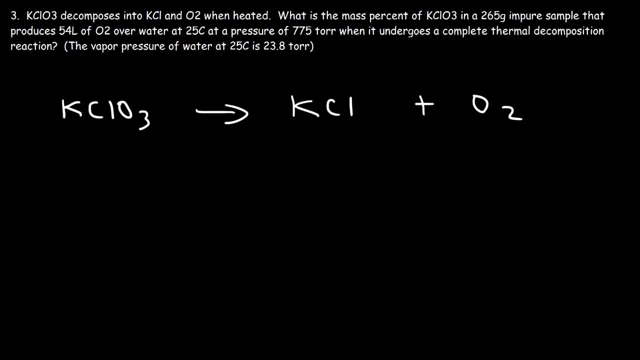 The least common multiple between two and three is six. So we need to get six oxygen atoms on both sides. So I'm going to put a two in front of KClO3, and a three in front of O2.. Now notice that I have two potassium atoms on the left. 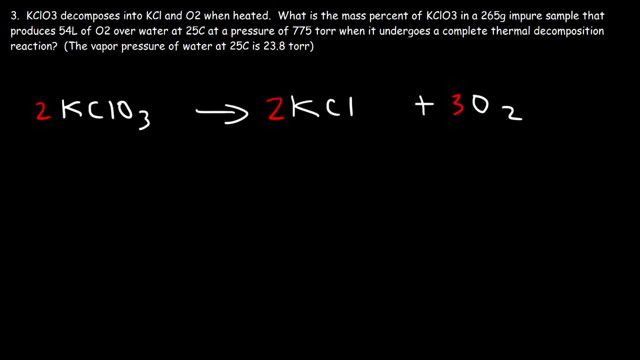 So I need to put a two in front of KCl, And now the reaction is balanced. So now, what is the mass percent of potassium chloride in a 265 gram unit? The mass percent of potassium chloride in a 265 gram impure sample that produces 54 liters. 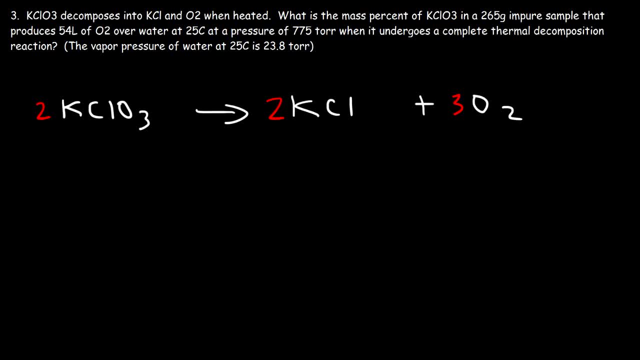 of O2 over water at 25 Celsius, at a pressure of 775 Torr, when it undergoes a complete thermo decomposition reaction. And we're given the vapor pressure of water at 25 Celsius, So let's write an expression that gives us the total pressure of all the vapors in this. 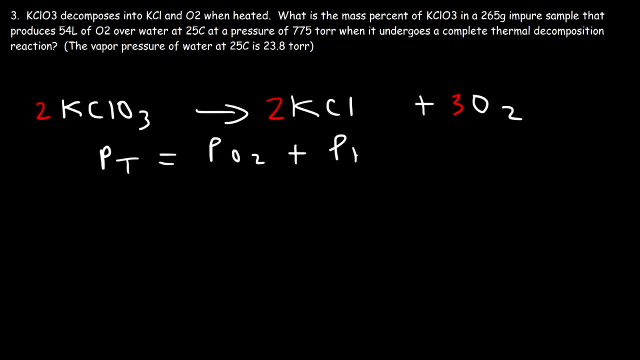 problem. So we have oxygen gas and water vapor. The total pressure is 775 Torr. We need to calculate the partial pressure of O2.. And the vapor pressure of water is 23.8 Torr, So we've got to subtract 775 by 23.8.. 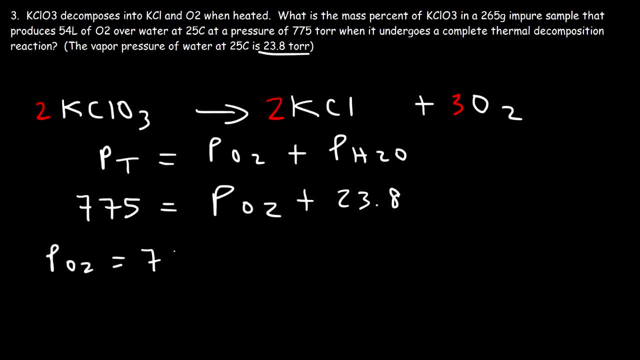 So the partial pressure of O2 is 751.2 Torr. But we need to convert that. That's to ATM, So we know that we've got to divide it by 7 stiffness, And so the partial pressure of O2 is 0.9884 ATM. 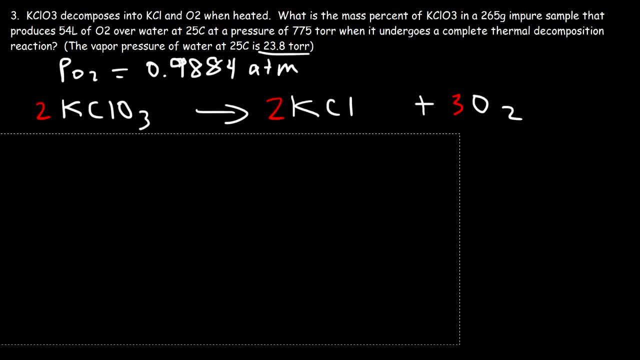 So using the partial pressure We have the productive fabric. Ok, Using the partial pressure of O2, we can calculate the moles of O2, and from that we can calculate the grams of KClO3 that was consumed in the reaction. 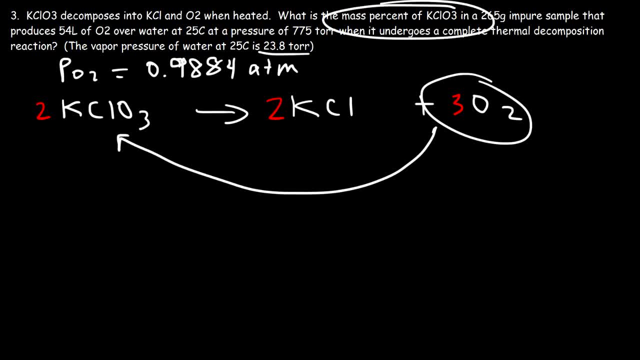 And once we have that, we can find the mass percent of KClO3 in the impure sample. So let's use the ideal gas law equation at this point. So the pressure is 0.9884 multiplied by the volume of 54 liters. here it is, and that's. 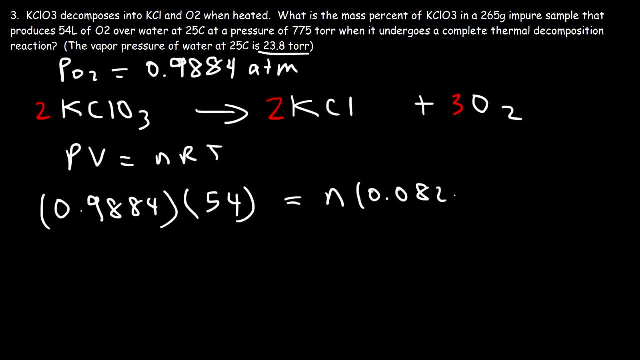 equal to N times R times the temperature. 25 plus 273 is 298.. 0.9884 times 54.. That's 53.984.. 0.3736 and 0.08206 times 298 is 24.454 times N. 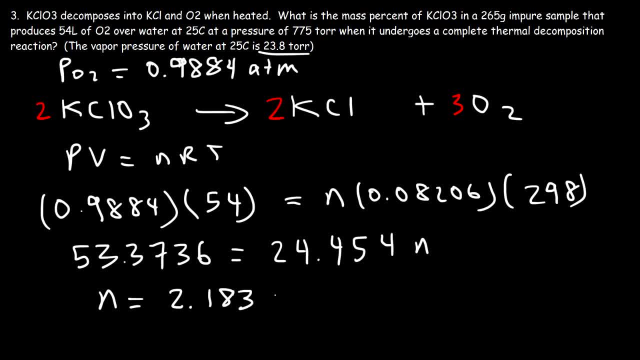 So N is about 2.183 moles. So now we can use this equation to calculate KClO3.. So let's start with 2.1 A3 moles of oxygen gas. Now the molar ratio between O2 and KClO3 is 2 to 3.. 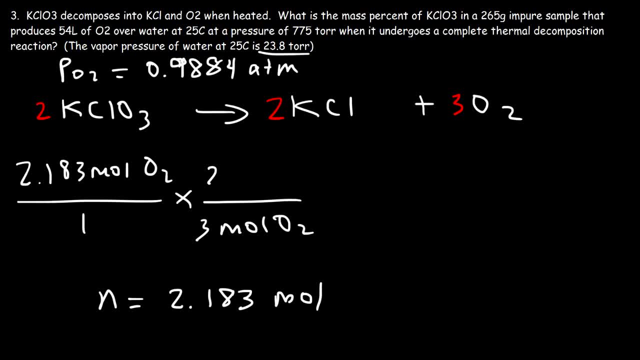 So for every 3 moles of O2 that's produced 2 moles of KClO3.. Okay, is consumed in a reaction. So now let's convert that into grams. So we need to find the molar mass of KClO3.. So we have one potassium atom, one chlorine atom and